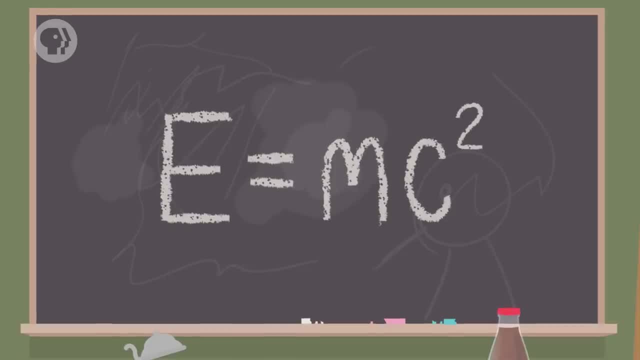 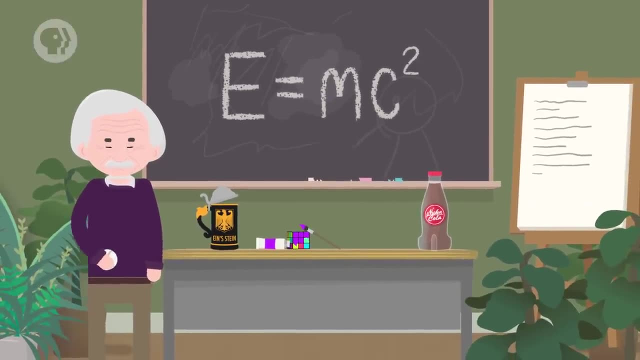 E equals mc2.. You hear it all the time, but what does it mean? During his study of special relativity, Albert Einstein found that mass and energy are equivalent and that they could be converted back and forth between one another. He described that relationship mathematically, saying that the energy of a particle is equal 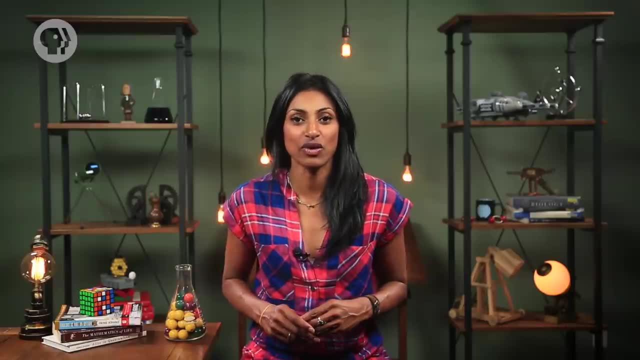 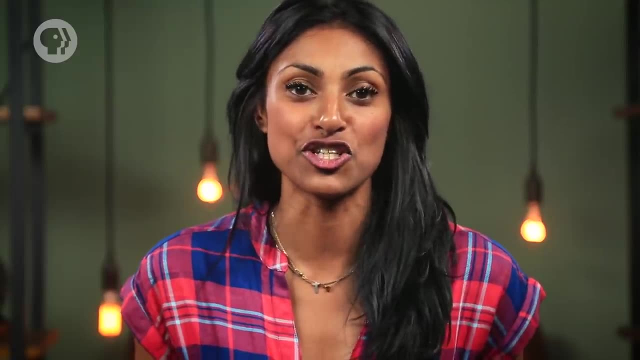 to its mass times, the speed of light squared. This mass-energy equivalence is critical to the study of nuclear physics, the study of the atomic nucleus. This is a branch of physics that introduces you to two of the four fundamental forces – one in which an element can turn into an entirely different element in just an instant. 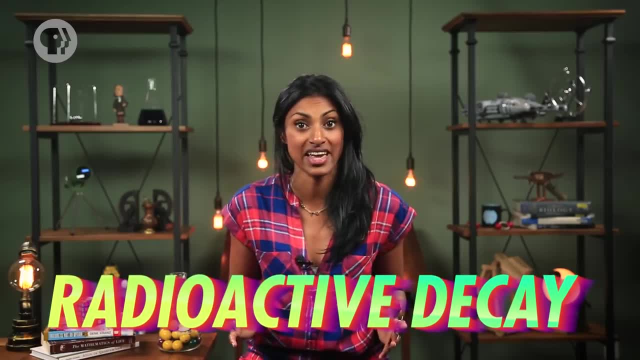 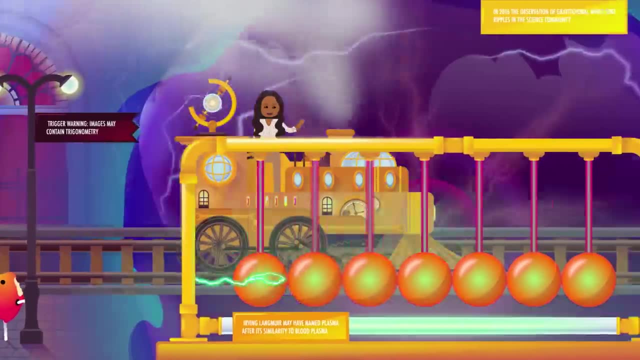 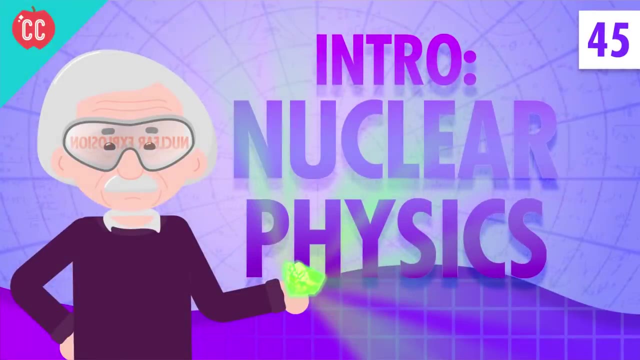 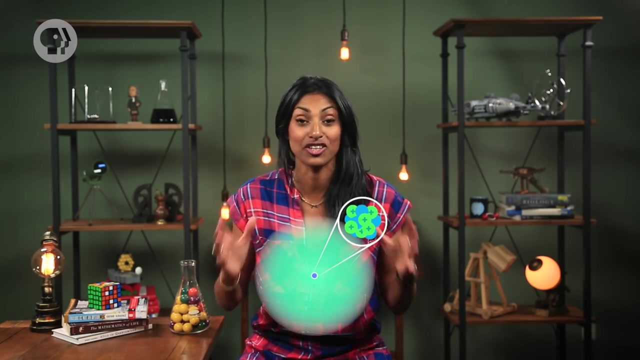 and one that has allowed us to unleash the incredible energy that's contained inside every atom. Before we can dive into the wonders of nuclear physics, we need to recall a little bit about the thing that makes it all tick – the nucleus. The nucleus of any atom consists of protons and neutrons. 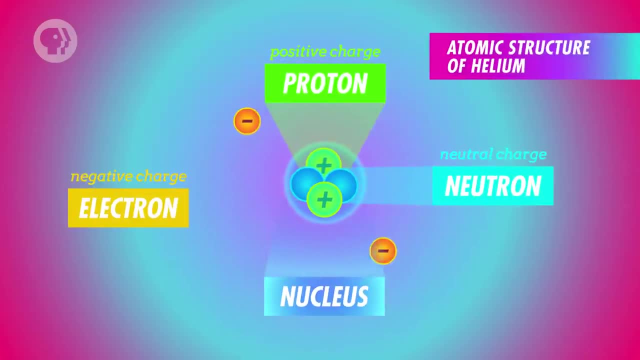 The proton is positively charged, while the neutron is electrically neutral, and both particles have nearly the same mass. With the exception of hydrogen, which only has a single proton in its nucleus, every element has both protons and neutrons. Because of this, we'll often refer to the two particles collectively as nucleons. 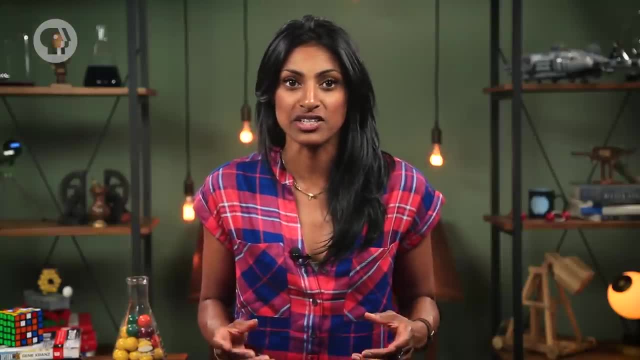 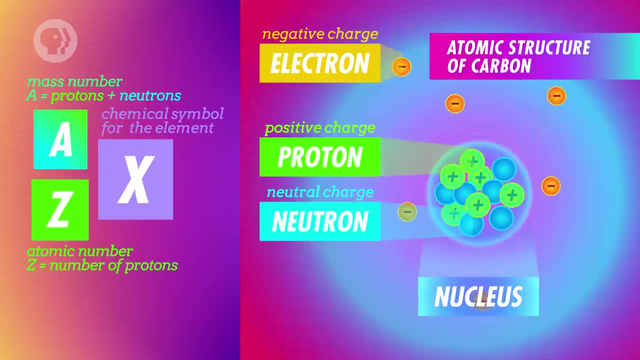 We can describe how many protons and neutrons are in an atom's nucleus using its atomic and mass numbers. An atomic number is how many protons are in a nucleus, which also determines what element the atom consists of. The mass number, meanwhile, is how many protons and neutrons combined make up a nucleus. 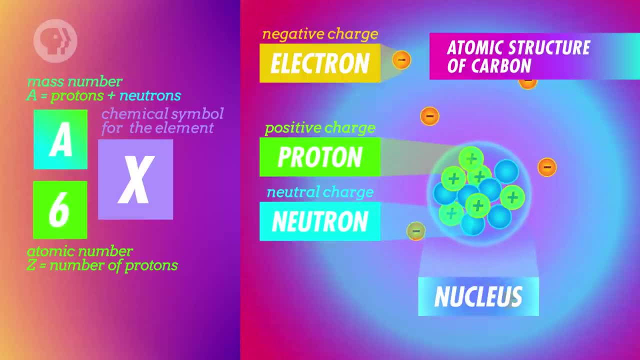 So if there are 6 protons and 6 neutrons in a nucleus, then its atomic number would be 6,, making it a carbon nucleus, and the mass number would be 6 plus 6, which is 12.. And if there were 6 protons and 8 neutrons, then it would still be a carbon nucleus. but 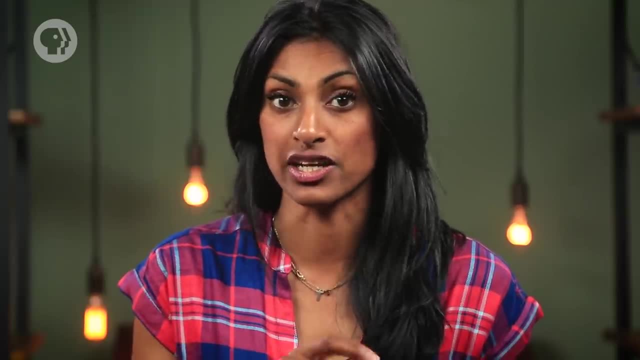 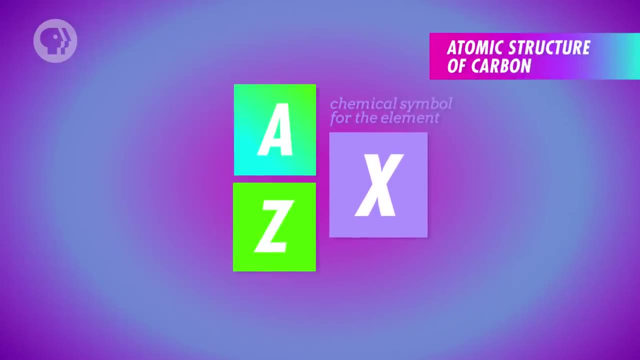 with a mass number of 14.. Let's put these carbon nuclei in nuclear notation To better show the differences between them. First we start with the chemical symbol for the nucleus, which is determined by its atomic number. Then on the bottom left of the chemical symbol, we write the atomic number, which will be: 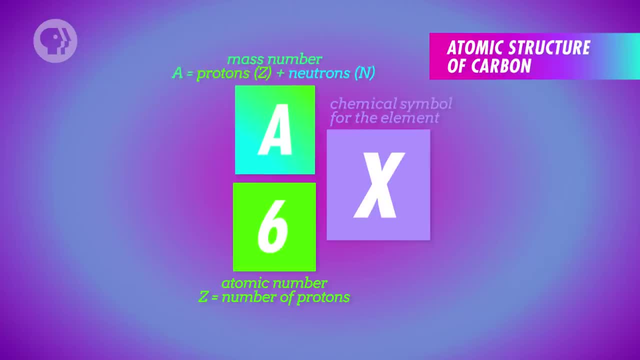 the same for both carbon nuclei – 6.. Finally, we write the mass number on the top left to signify how many protons and neutrons there are in the nucleus. So for our carbon atom with 6 neutrons we'd take the carbon chemical symbol, a capital. 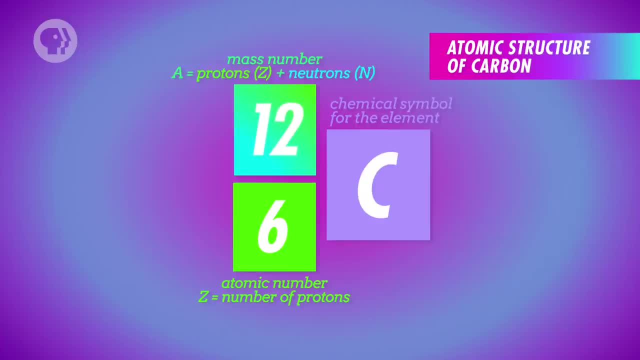 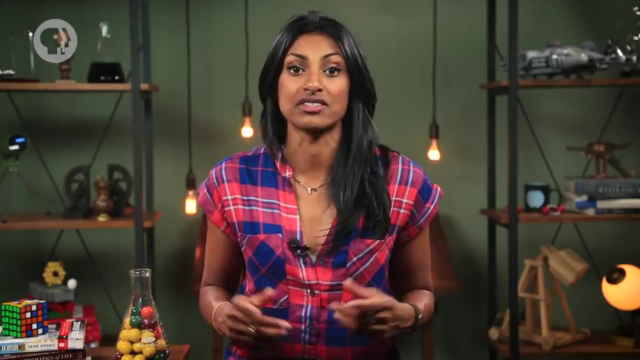 C and write the atomic number 6 in the bottom left and the mass number 12 in the top left, The upper left mass number becomes 14.. Any two nuclei that have the same atomic number but different mass numbers are known as isotopes. 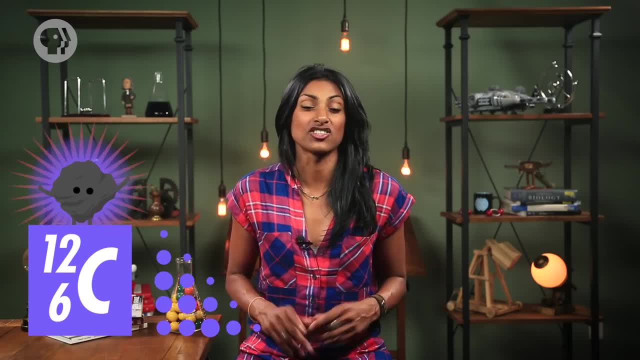 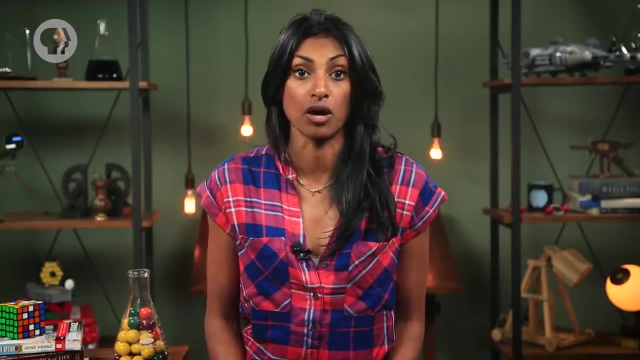 with most elements having one isotope that's more common than the others. For instance, 99% of the carbon on the Earth is carbon-12,- carbon with a mass number of 12.. Only a tiny fraction of all carbon on Earth is carbon-14,, since carbon is most stable. 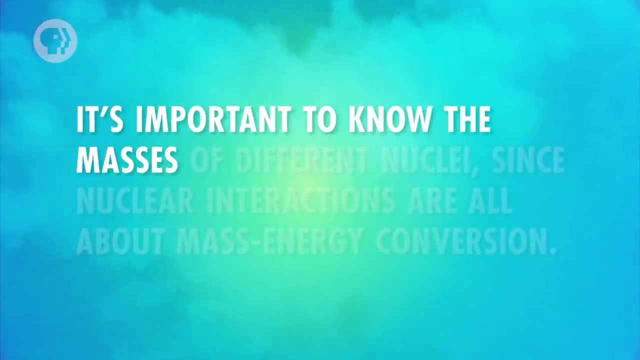 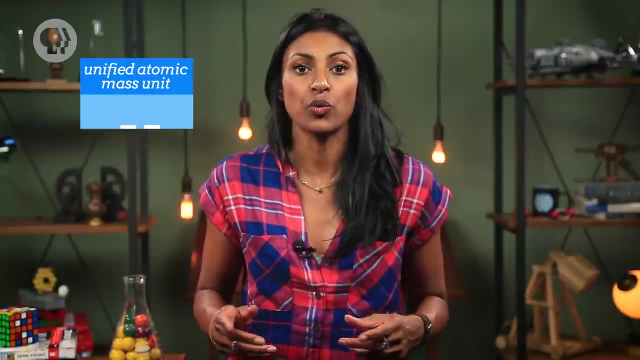 when the number of protons equals the number of neutrons. It's important to know the masses of different nuclei, since nuclear interactions are all about mass-energy conversion. To quantify the mass of a nucleus, we use the unified atomic mass unit. written just. 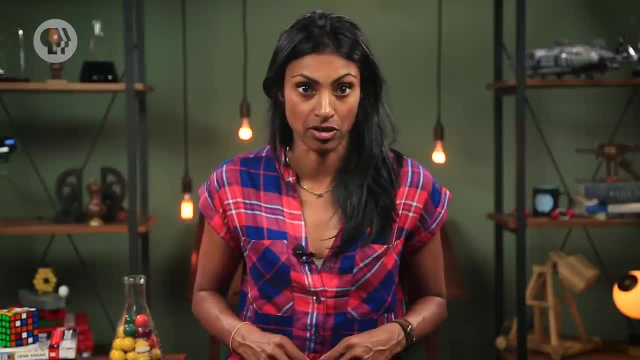 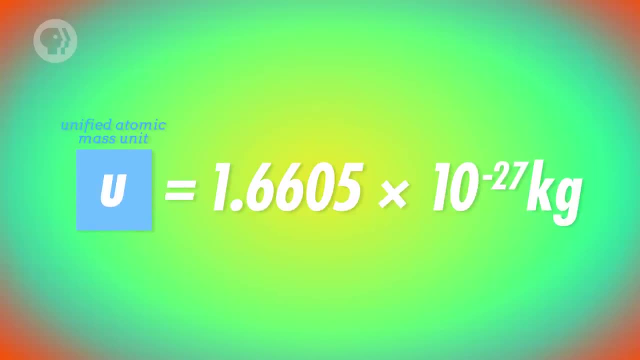 as a small u. A single neutral carbon-12 atom, for example, equals exactly 12 unified atomic mass units. This means that one unified atomic mass unit is equal to 1.665 times 10, to the negative 27th kilograms. 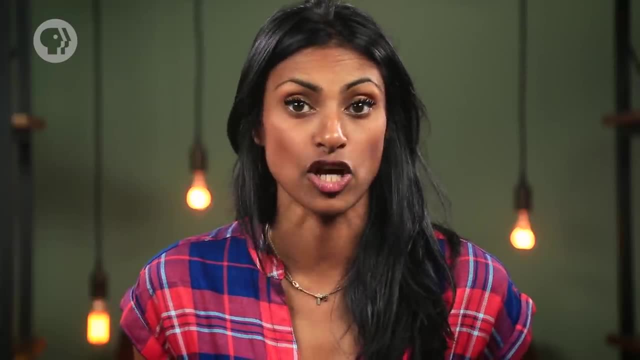 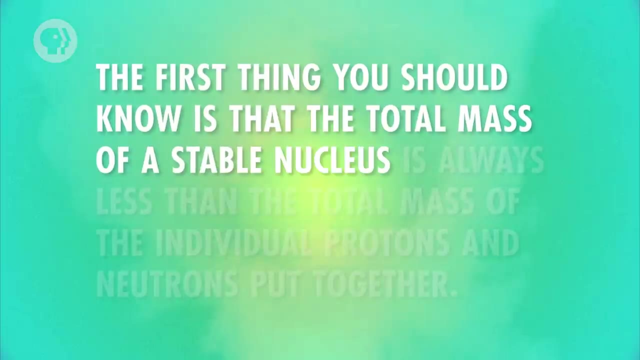 OK, now that we have a notation for describing elements and their isotopes, we can talk about the energy associated with a nucleus and its bonds. The first thing you should know is that the total mass of a stable nucleus is always less than the total mass of the individual protons and neutrons put together. 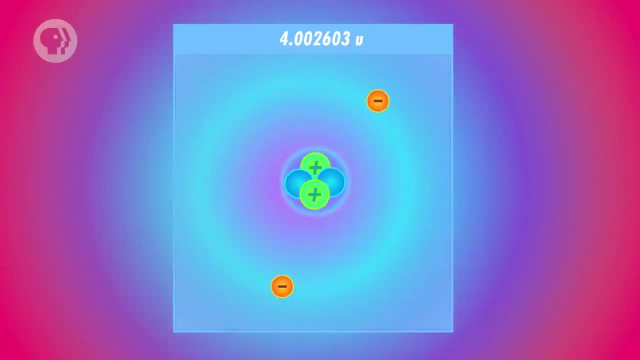 For instance, the mass of a neutral helium atom is 4.00603 unified atomic mass units, But two neutrons and two protons, the component parts of a helium atom, taken together, have a mass of 4.032980 unified atomic mass units. That means that the nucleus of a helium atom has 0.03037 unified atomic mass units less mass than its component parts. How can that be? Well, that difference in mass is equal to an amount of energy, specifically the total binding energy of the nucleus. 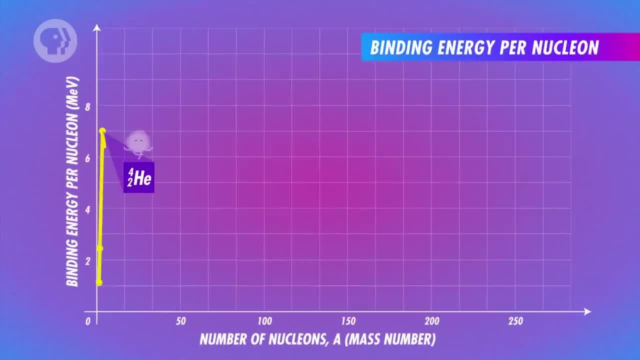 That binding energy is how much energy you would have to add to the helium atom in order to break apart its nucleus. The amount of energy required to break up a nucleus into its component particles gets larger as the atomic number increases, with iron having one of the highest binding energies. 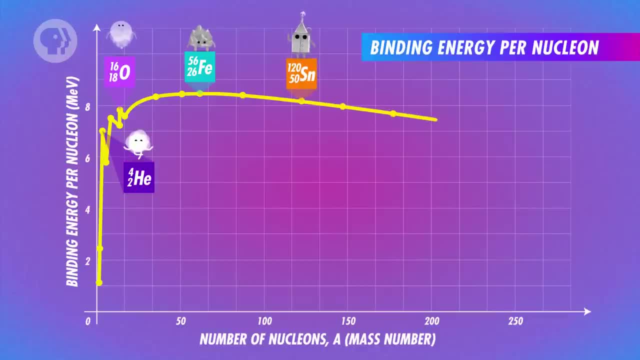 per nucleon, But while the total binding energy still increases, for a nuclei larger than iron, the binding energy per nucleon in fact decreases. This means that the total binding energy of the nucleus is less than the total binding energy of the nucleus. 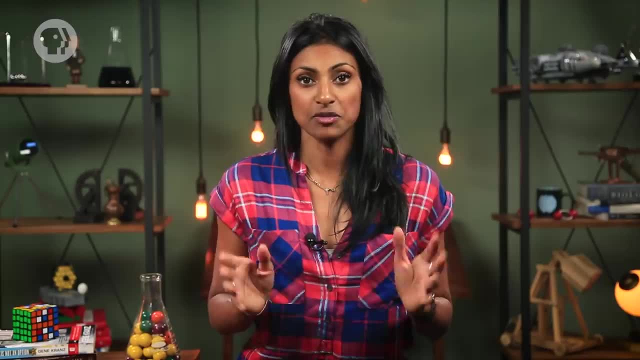 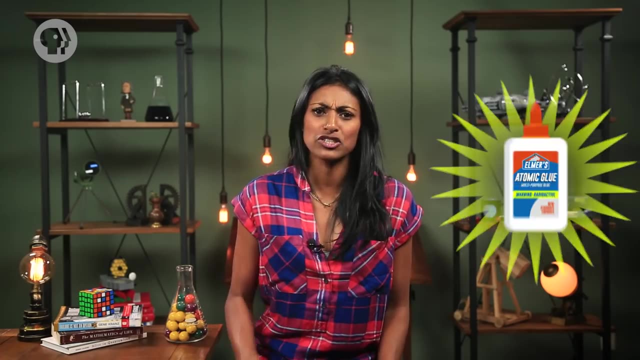 This means that very large nuclei are not held together as strongly as small nuclei. Since binding energy accounts for the missing mass. you can calculate it using. you guessed it. e equals mc squared. Now you might be wondering how a nucleus is held together in the first place. 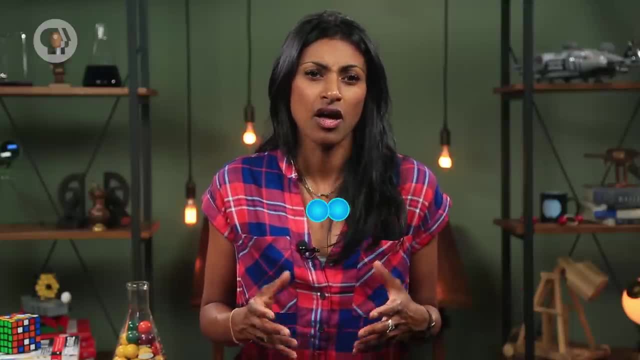 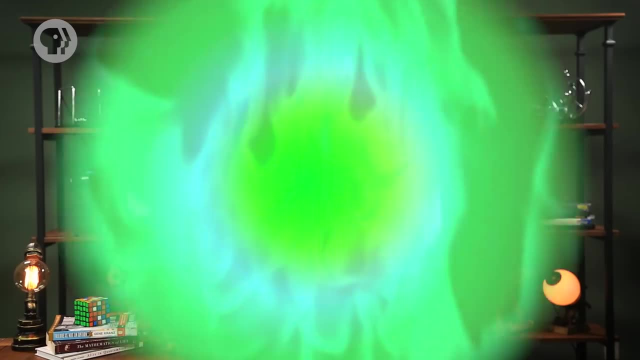 You've got neutral neutrons having no problem getting close to one another. But what about all the positive protons? Shouldn't the repulsive electric force keep them apart? Well, one of the four fundamental forces of physics is the strong nuclear force, an attractive 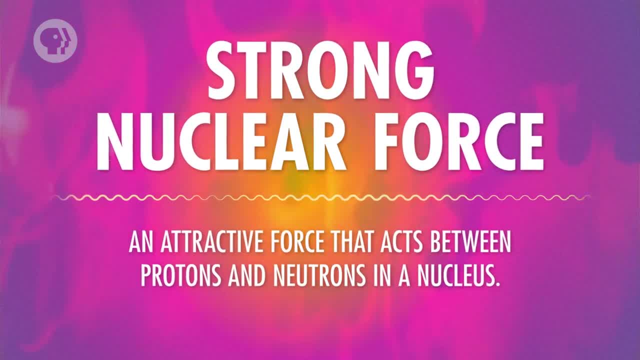 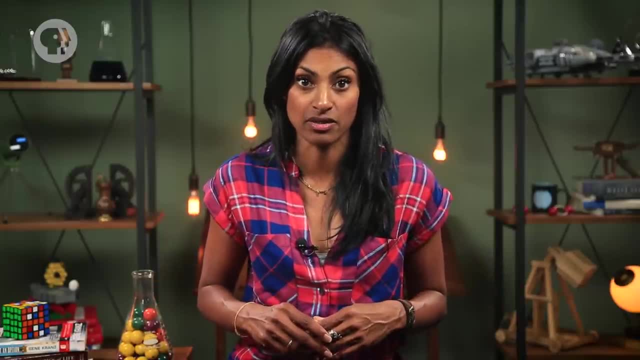 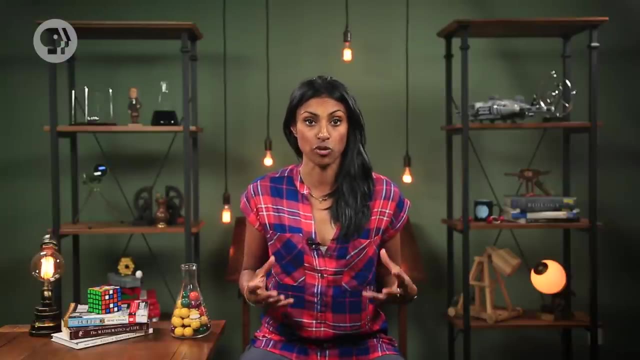 force that acts between protons and neutrons in a nucleus. This strong force is substantial enough to overcome the repulsive force between protons, but it only acts over very small distances, while the electric force acts over longer distances, Since the strong force only works across such tiny distances. larger atoms with high atomic 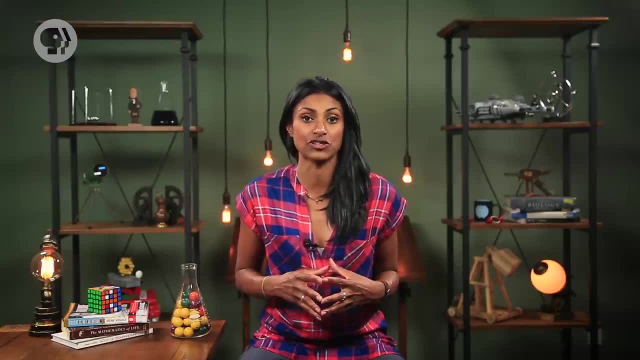 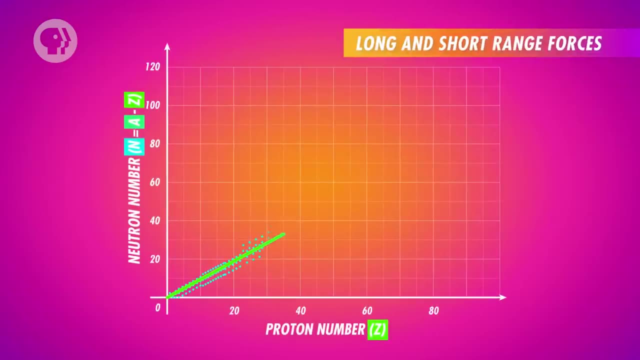 numbers actually require additional neutrons to overcome the electromagnetic force and maintain stability within the nuclei. Those extra neutrons are necessary for atoms with atomic numbers higher than 30 or so, as you can see in this chart relating the number of neutrons to the number of protons. 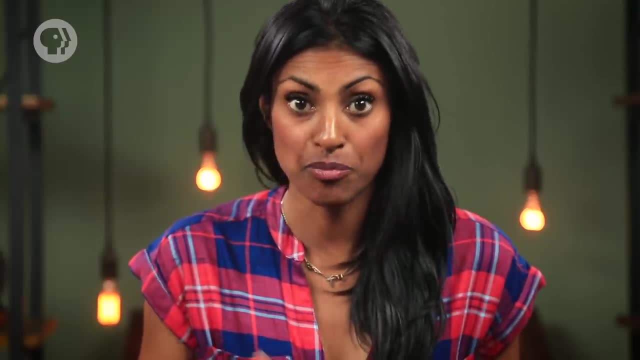 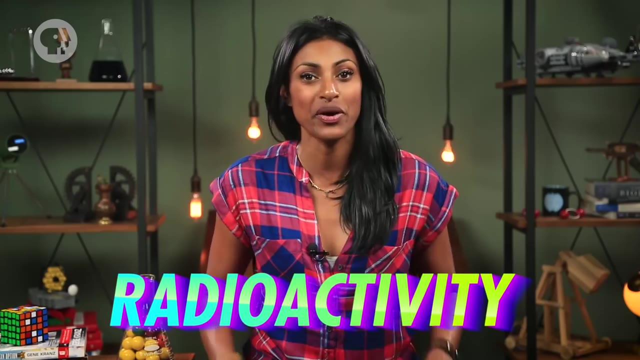 in a stable atom. When a nucleus is unstable, it can break down into a more stable state. This decay of unstable nuclei, accompanied by the emission of energetic particles, is known as radioactivity. Natural radioactivity was first discovered by Henri Becquerel, who observed how a chunk 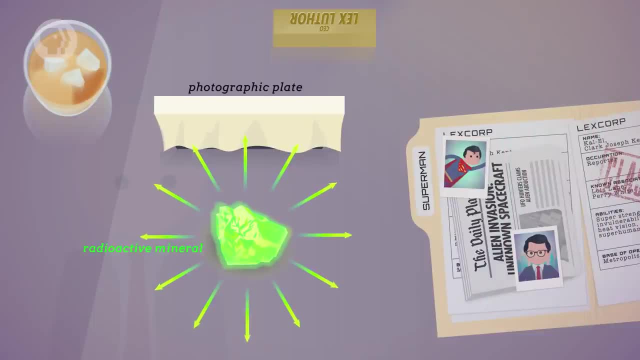 of mineral that contained uranium affected a photographic plate that was covered up by paper. Even though the paper was blocking out visible light. the radiation from the uranium penetrated the paper and left its mark on the plate. Later, scientists studied such decays and categorized the emitted rays or particles. 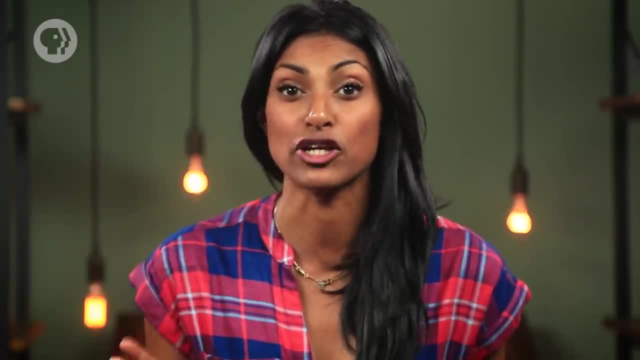 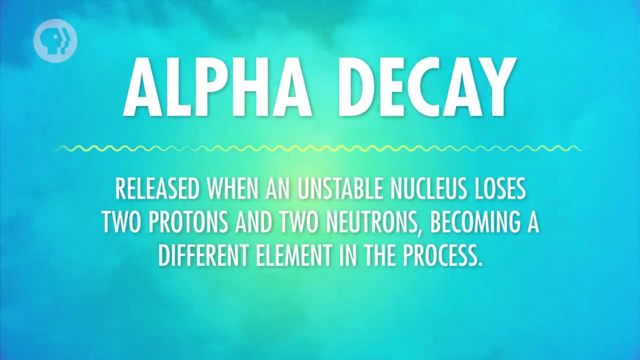 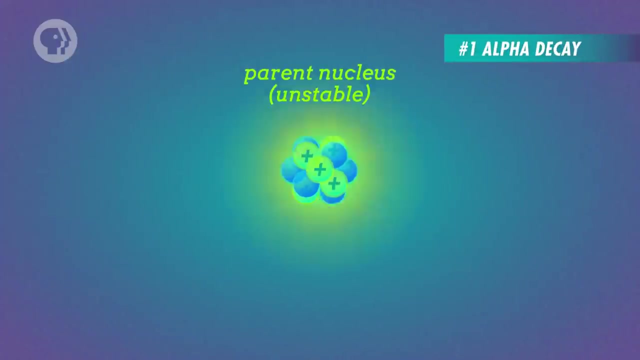 in a stable atom. In the first case, there's alpha decay, which is released when an unstable nucleus loses two protons and two neutrons, becoming a different element in the process. In alpha decay there's a parent nucleus, which is the original unstable nucleus, and 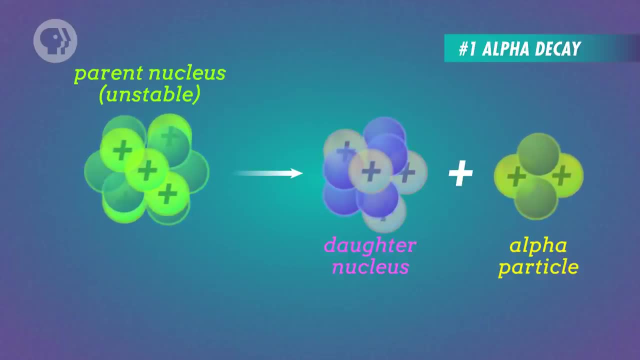 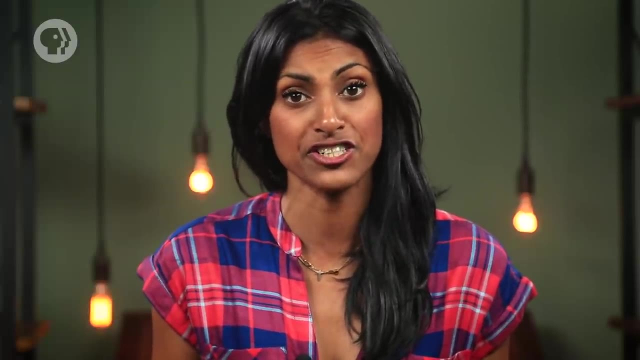 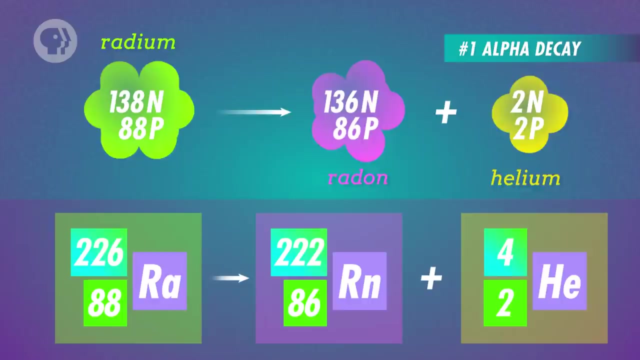 it decays into a daughter nucleus and an alpha particle, which is actually just the nucleus of a helium atom. This decay occurs because the parent nucleus is too large and the strong force is no longer sufficient to hold all the nucleons together. For example, if the parent nucleus is radium, it would decay into radon and emit a single. 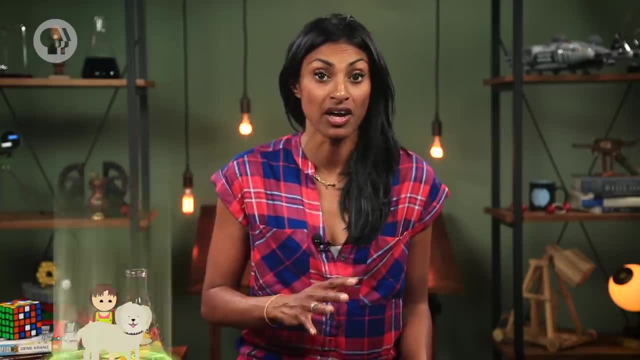 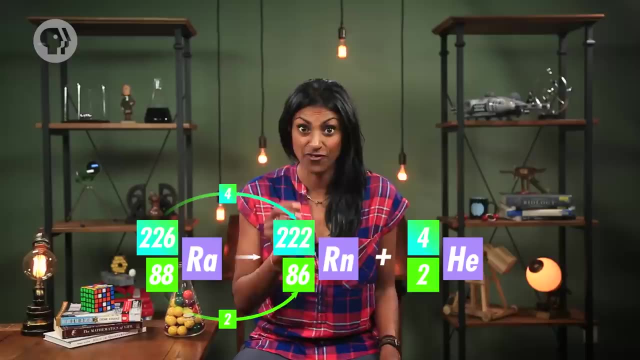 alpha particle. The process of the nucleus changing from one element to another is known as transmutation. Note that the atomic number of radon is just two units less than that of radium and the mass number is four less than radium's. 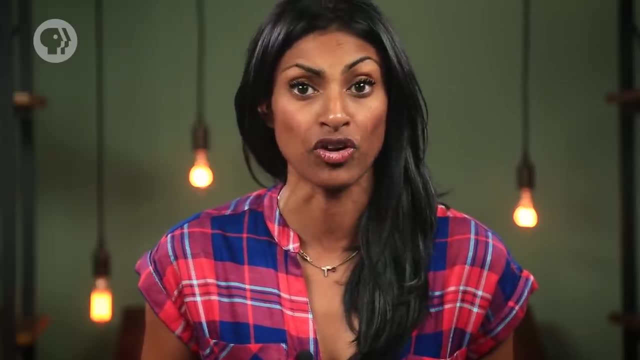 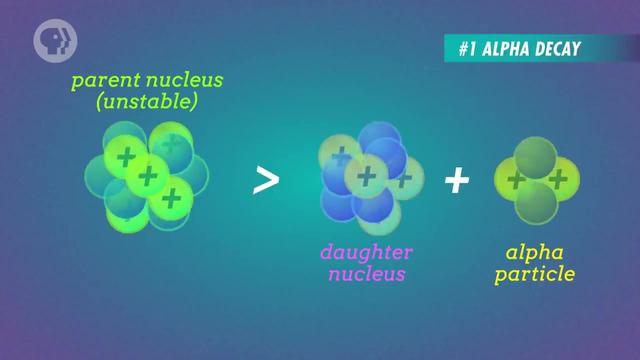 In alpha decays. the sum of the atomic and mass numbers are always equal on either side of the equation. But even though those numbers of nucleons add up, remember mass and energy are equivalent. So the products of this reaction always have less total mass and the mass of the nucleons. 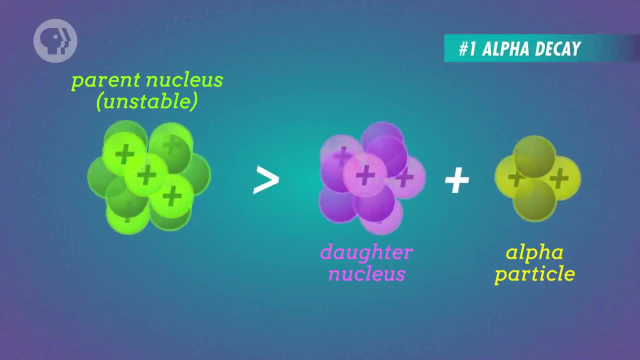 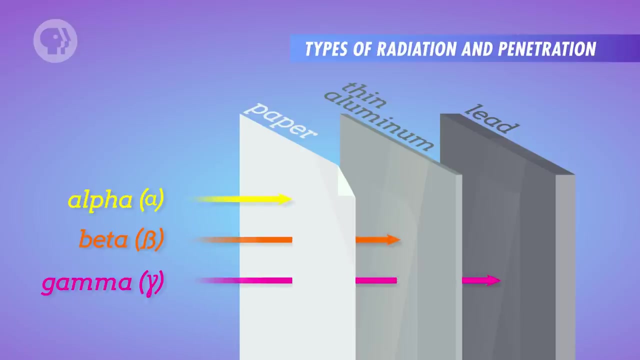 are equal. They have less total mass, as measured in unified atomic mass units, than the parent nucleus has The rest of the mass turned into kinetic energy, and the kinetic energy released in nuclear reactions is what's used to generate nuclear power. But alpha particles have the least penetrating power of the three groups – they're barely 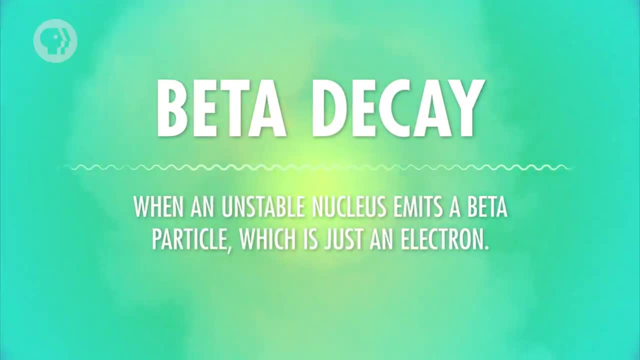 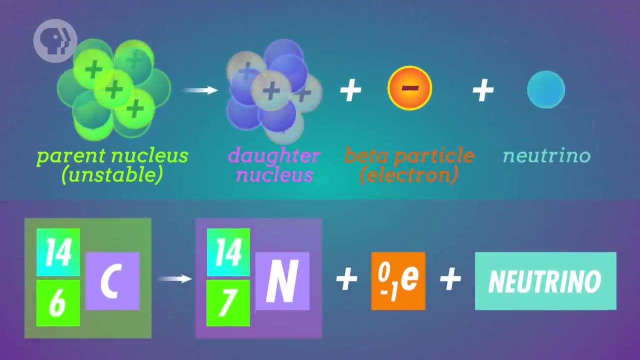 able to pass through a piece of paper. The second type of decay that can occur is beta decay, when an unstable nucleus emits a beta particle, which is just an electron. You'll see that whenever an electron is produced, so is a neutrino. 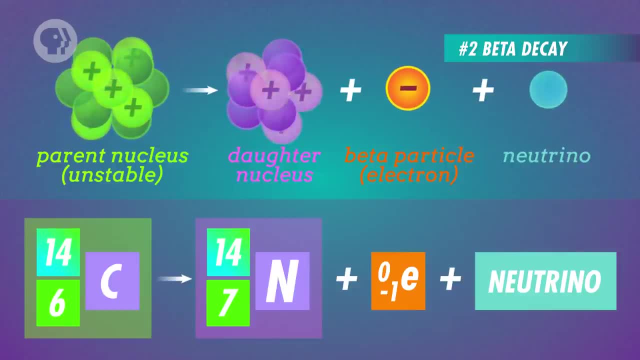 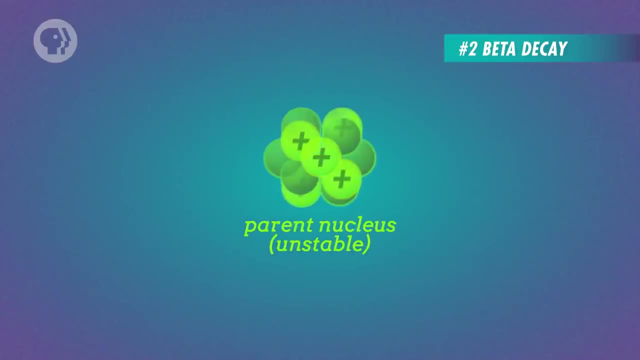 A neutrino is a particle that is not a neutron. A neutrino is a particle with a very small mass that is electrically neutral. Its existence is inferred from the conservation of energy. For example, when a nucleus at rest decays into two fragments, it should give each fragment. 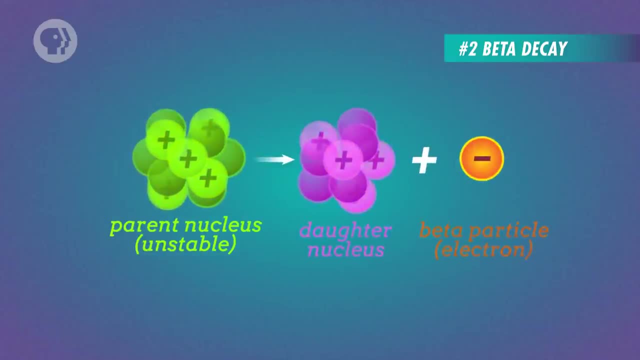 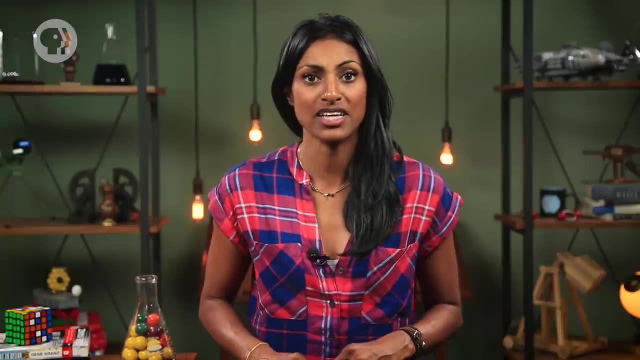 the same amount of momentum. If the nucleus decayed into the daughter nucleus and an electron, the electron would always have the same momentum and the same energy, But electrons from beta decay have been found to have energies that vary greatly. This suggests that a third particle must be carrying away the rest of the energy and 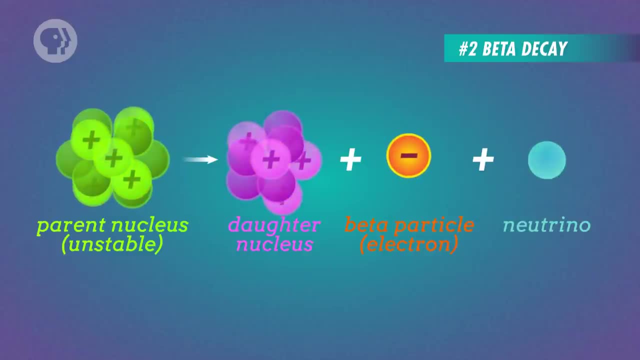 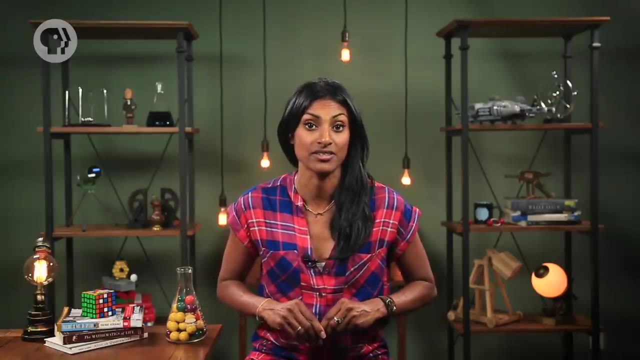 experiments have confirmed that these tiny neutrons are the same energy. Now, a unique part of beta decay is that no nucleons are emitted during the decay process. Instead, one of the neutrons changes into a proton, and to compensate for the change, 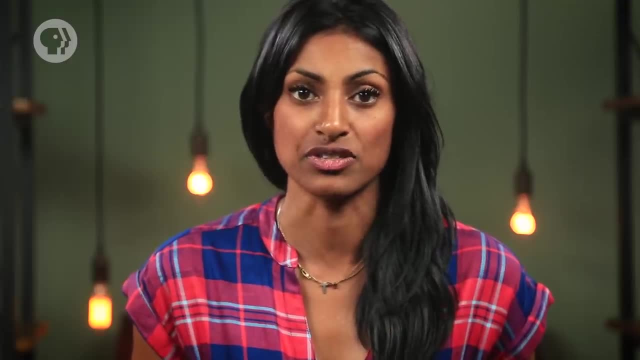 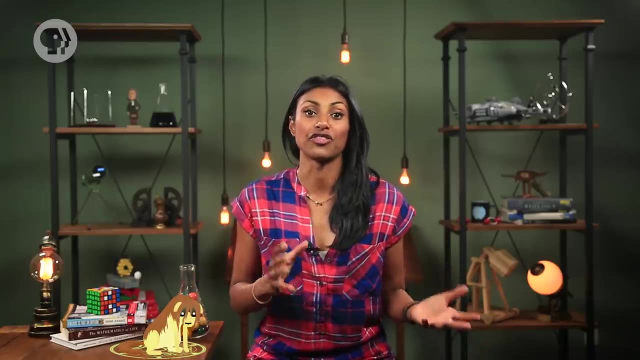 in charge. the neutron emits an electron, And although these electrons come from nuclear decay, they're the same kind of electrons that orbit a standard nucleus. Once the neutron changes into a proton, the nucleus changes from one element to another. again an instance of transmutation. 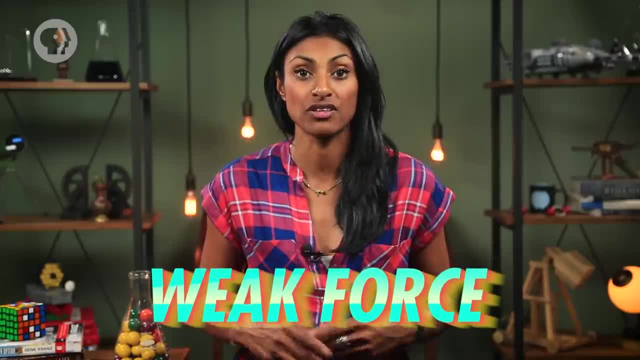 And beta decay is caused by the change in charge of the electron. The electron emits an electron. This is caused by the fourth fundamental force, the weak force. While the strong force acts on nucleons, the weak force alters quarks. the fundamental 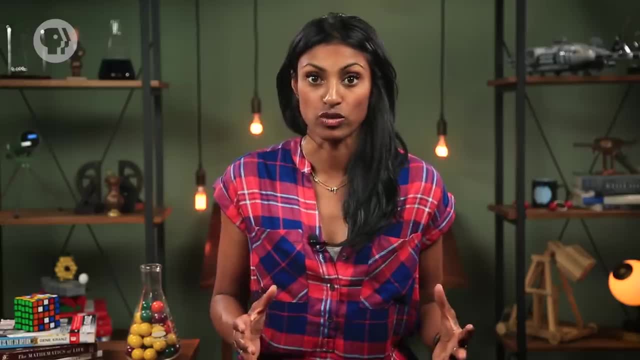 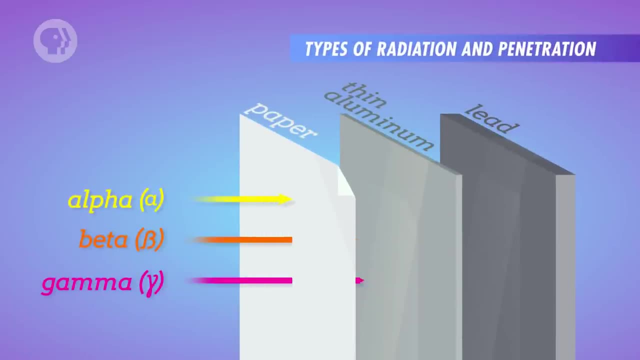 particles that make up both protons and neutrons. By converting quarks of one type into another, the weak force causes the neutron to turn into a proton. As for their penetrating power, beta particles are typically stopped by a few millimeters of aluminium.